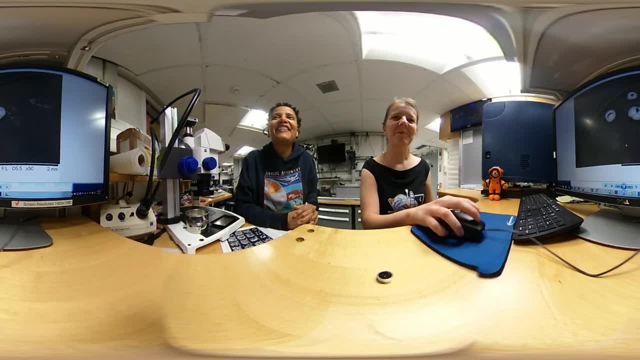 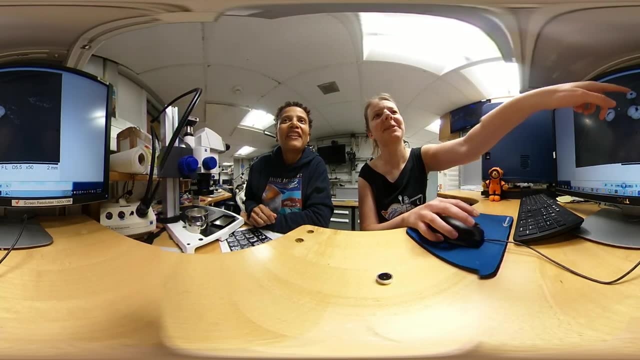 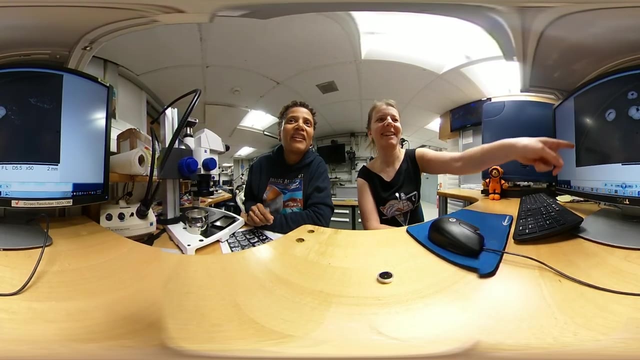 the screen and we can see exactly all the details of the shells. so this one is magnified about 50 times. so you see those three little blobs, they are the planktic forums that I just showed you on the stub. and then this big line here- that's the eyelash that was also on the stub, just for scale. Wow, so they are. 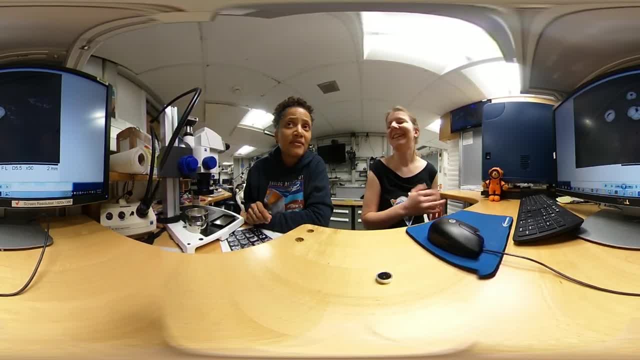 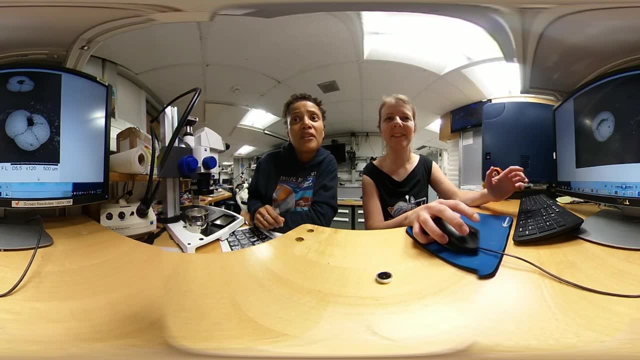 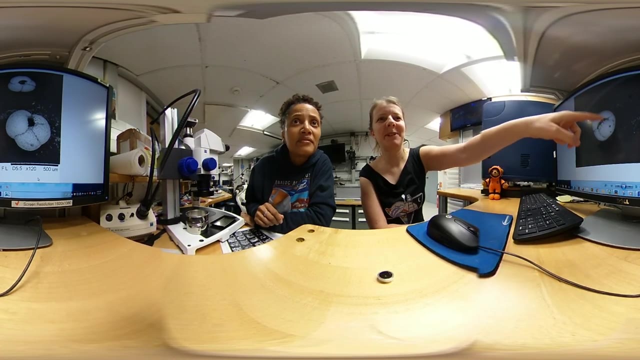 really small. they're really really small. they're about the size of a grain of sand, and then we can zoom in on that a lot closer. so this is a hundred and twenty times magnification. so you can see, this eyelash is getting really, really broad, mm-hmm. and now we can see a little bit more detail on the shells. so we see that. 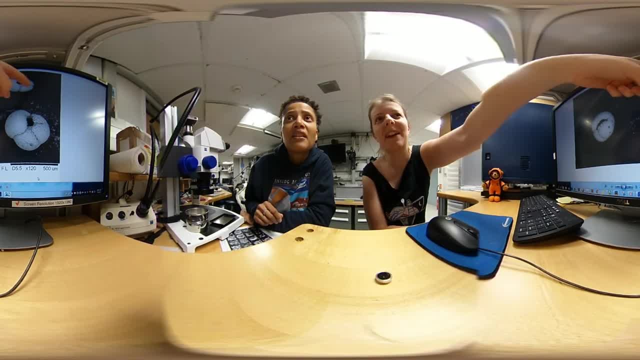 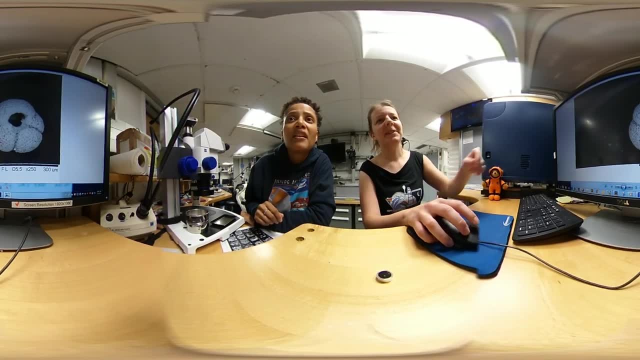 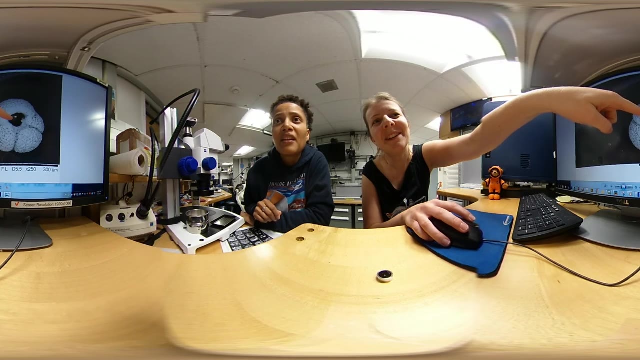 they've got a large opening in the middle, some smaller pores on the wall structures of their shells, and they're zooming in even closer. so again, this is the eyelash. you can see how small this thing really is. you can see a little bit of the internal structure of the chambers and we can see some, some of 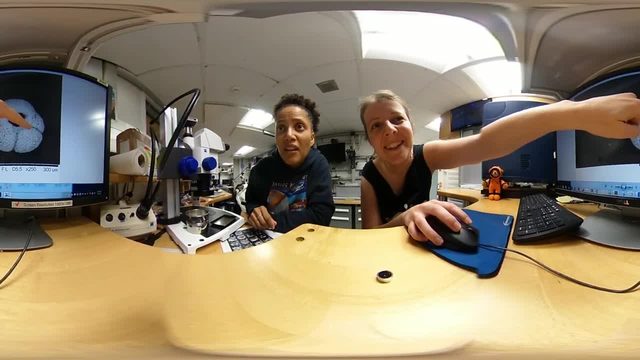 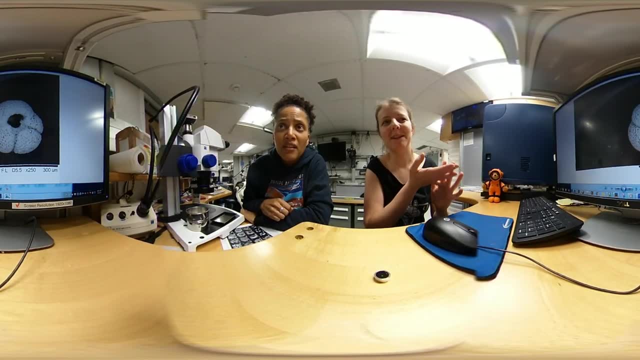 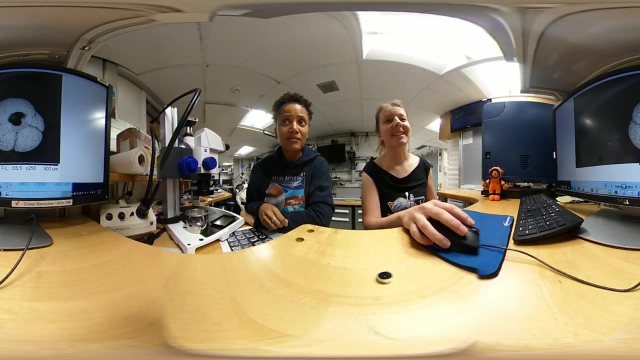 the pores really nicely. and then there's these tiny gray dots on them. what are those? so they're not part of the shell, they're just bits from the sediments that have been sort of accumulated to the inside of the shell and they're not Accumulating on the on the forums as they were preserved in the sediments. So even smaller bits, Yes, Yes, loads for all of it. 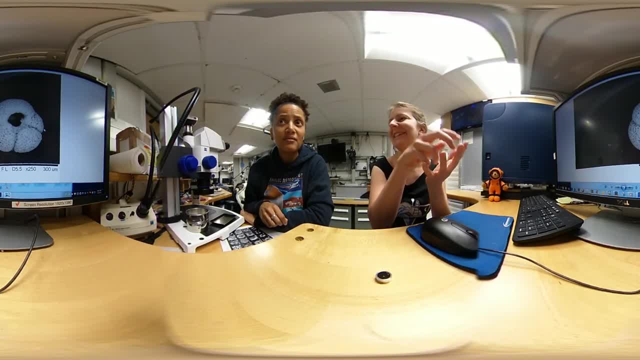 And sometimes we can see Fossils in this stuff that are a thousand times smaller than this forum. Wow, that's super small. So they're so small that you can't see them with the naked eye. even with just a normal light microscope You wouldn't be able to see them, But with this microscope we can. so if we zoom in a little bit closer, 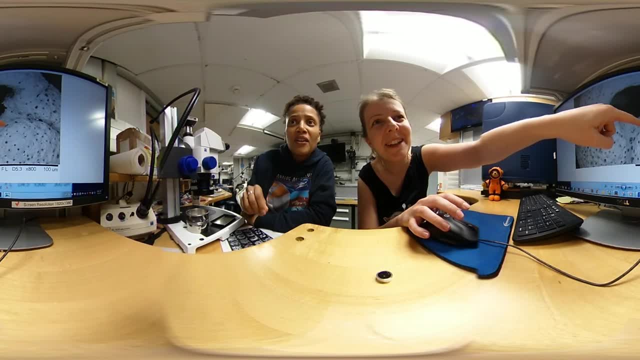 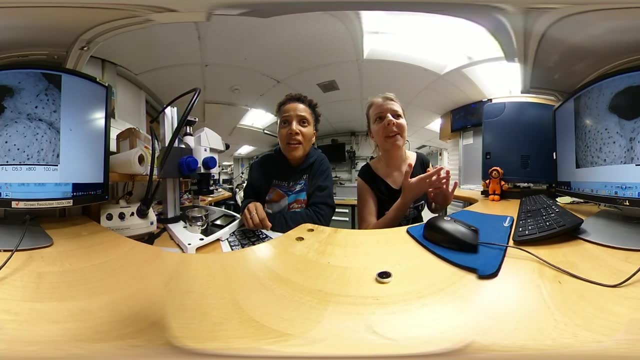 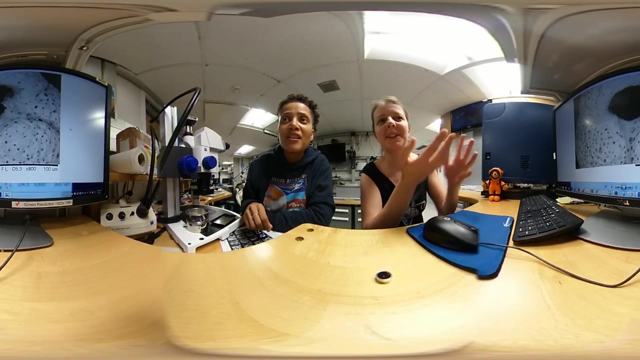 You can see all these little gray specks that actually made up these tiny little plates. Wow, so these are all from a group of Microfossils called coccolithophores. They built these sort of spherical structures made up all these tiny little plates that are all interlocking and 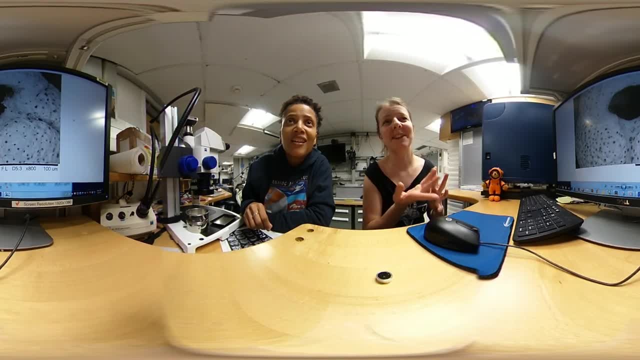 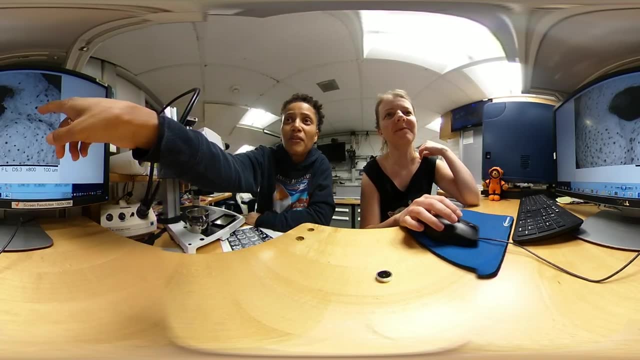 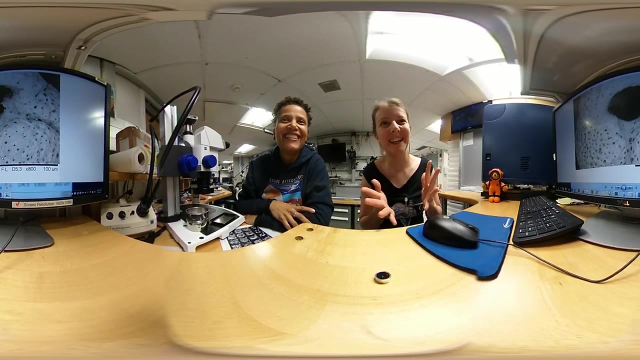 These are a couple of micrometers across, So they're really, really small. You really need advanced microscopes to be able to see them. Wow, So fossil parts of a fossil on top of another microfossil, Exactly. Yeah, Going from small to really small.